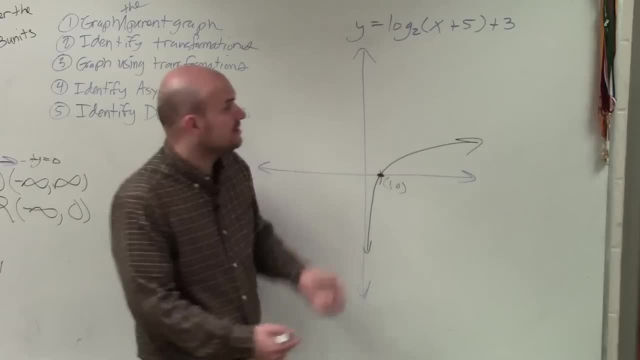 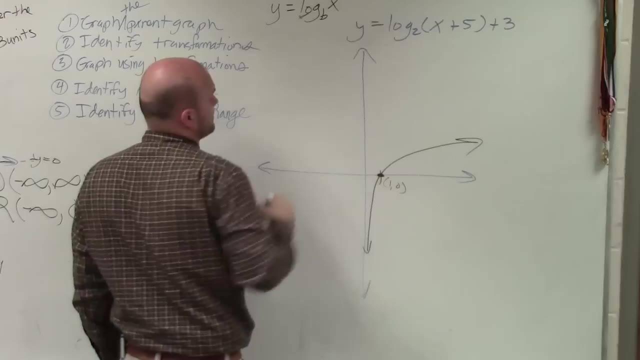 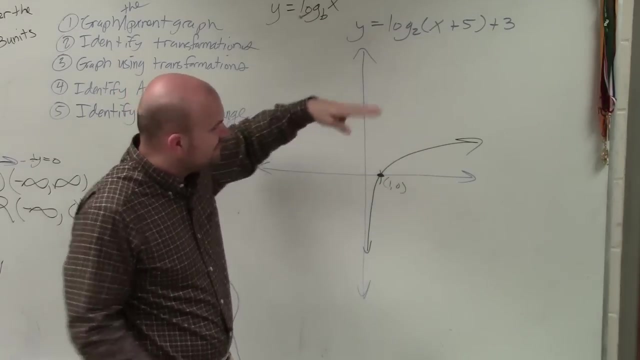 Wait, I want to know what the base is. Wait, I want to know what the base is. Always, unless there is like a number: y equals log base b of x, As long as it looks like in this format, b is going to affect how sharp the graph curves right Or how wide it goes. However, 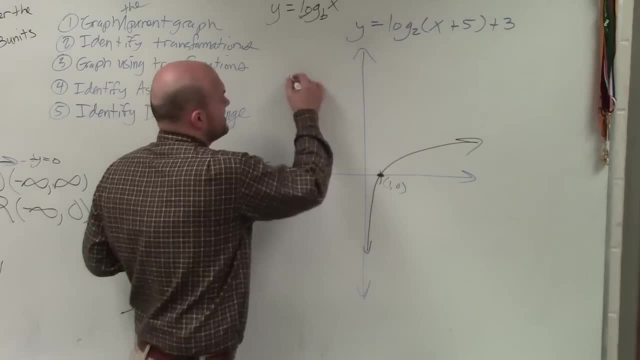 it's always going to cross at 1 comma 0.. Just like this: If I said y equals b to the x, that graph is going to be 0.. And if I said y equals b to the x, that graph is going to be 0.. 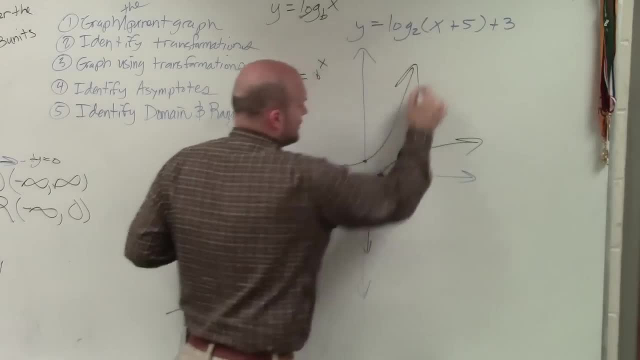 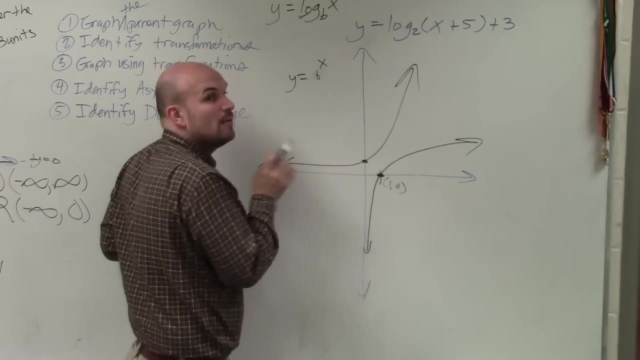 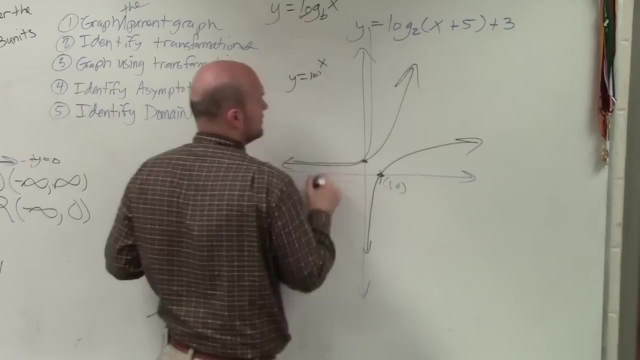 So that graph always crosses at. that graph always looks like this, Always. It's never going to cross at a different value. However, the shape of it could be different, Like, for instance, if I say this is 100, then the graph is going to go like this: If I say that's 1 half, then the graph is going to go like that: 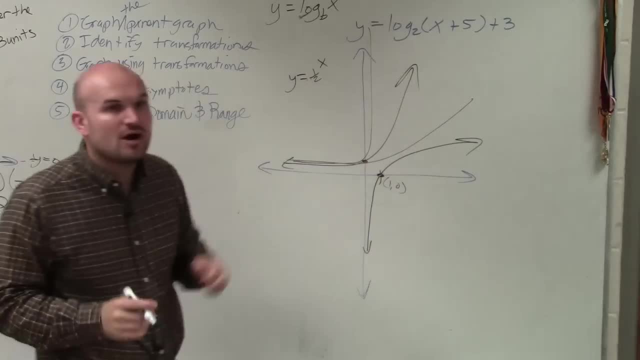 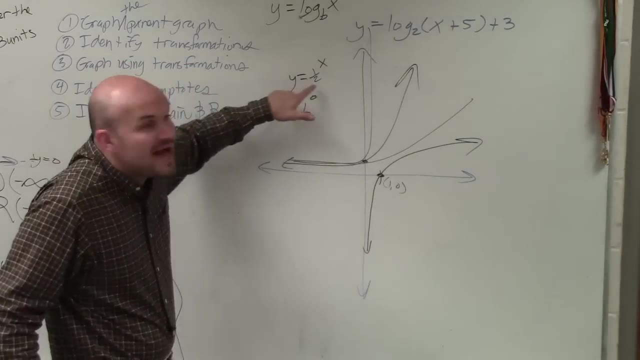 So the shape of it will be different, but it's always going to cross at 0.. Why? Because what is any number raised to the 0? Narrow power, 1.. So it doesn't matter what b is, It's always going to cross at 1.. 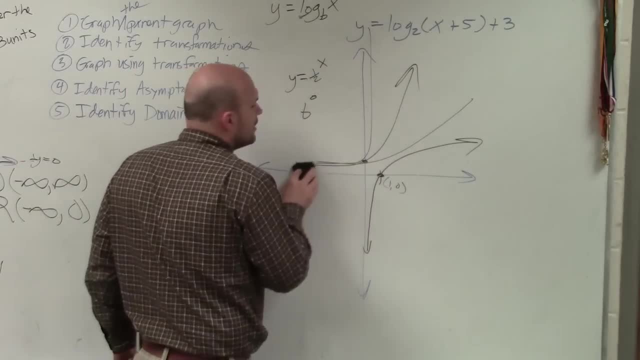 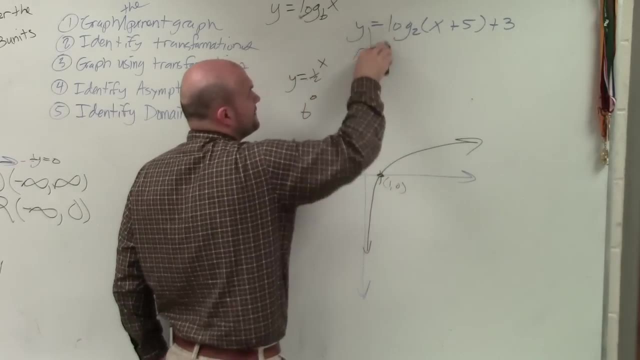 How do you know when to like turn a rule to start Right now, I'm not asking you guys to worry about that with logarithms. So the way that we found out to do if it's really sharp or not for exponential was to use a table of values. right, You plotted. 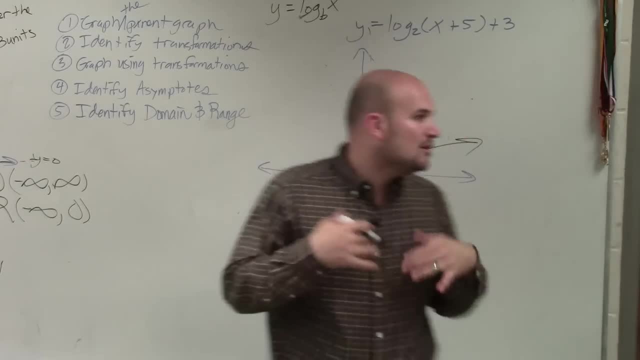 points and that's how we determined if it was sharp or great For logarithms. right now I'm not really concerned. I'm not going to be concerned with the table. I just want you guys to understand that I'm not going to be concerned with the table. I just want you guys to understand that. 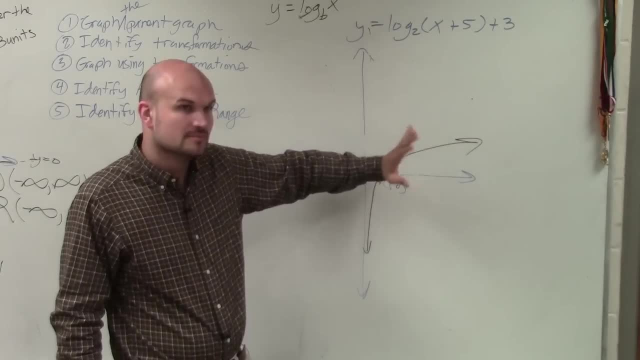 you guys to understand what the general format of the graph looks like. That's why I was saying I was kind of easy to you guys, I left you off the hook. I just said, hey, sketch what the shape of the graph is. 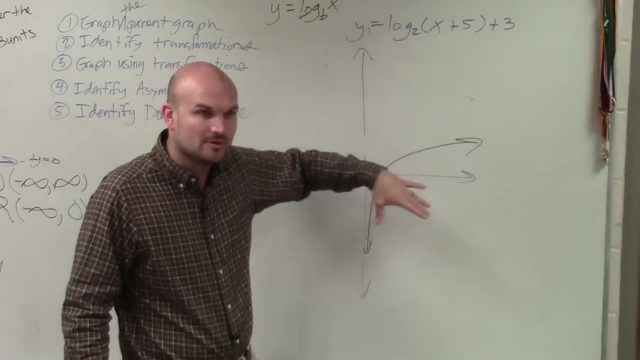 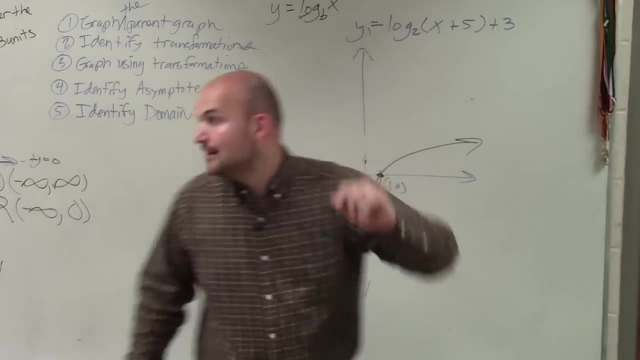 Because once we learn about logarithms you'll learn how to do a table. But for right now, just know what the shape of the graph looks like and know that it graphs across that 1 comma 0 when it's in that format. 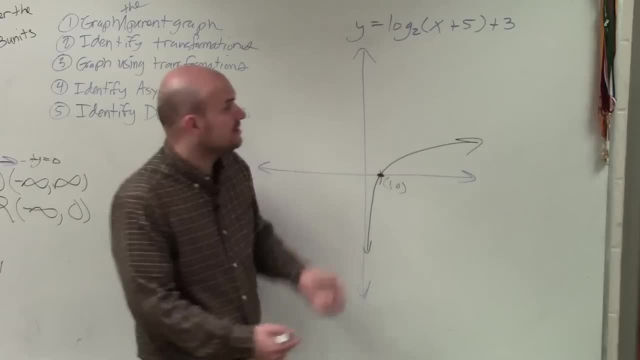 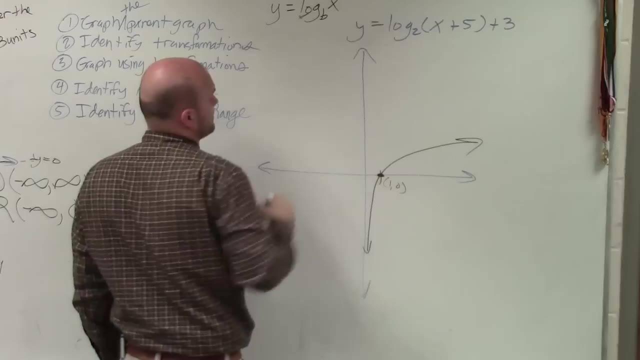 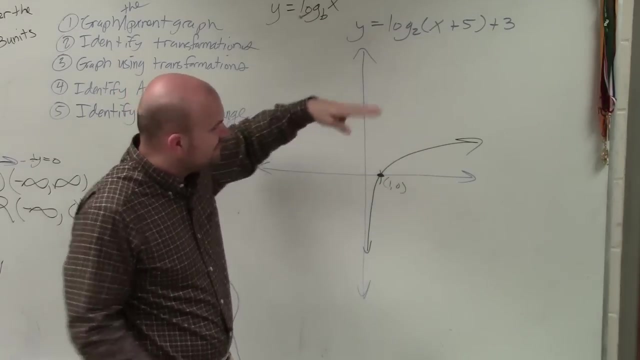 Wait, I want to know what the base is. Wait, I want to know what the base is. Always, unless there is like a number: y equals log base b of x, As long as it looks like in this format, b is going to affect how sharp the graph curves right Or how wide it goes. However, 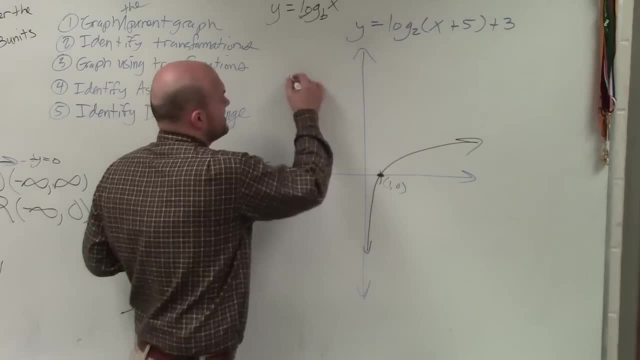 it's always going to cross at 1 comma 0.. Just like this: If I said y equals b to the x, that graph is going to be 0.. And if I said y equals b to the x, that graph is going to be 0.. 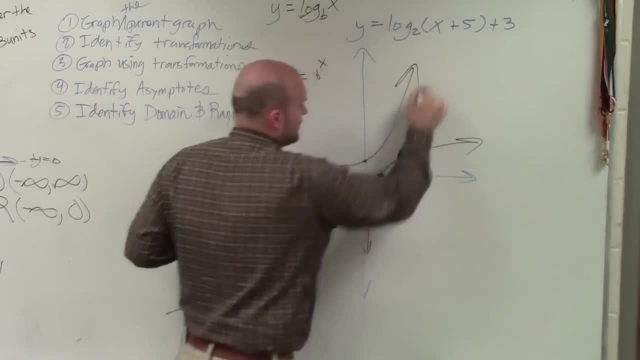 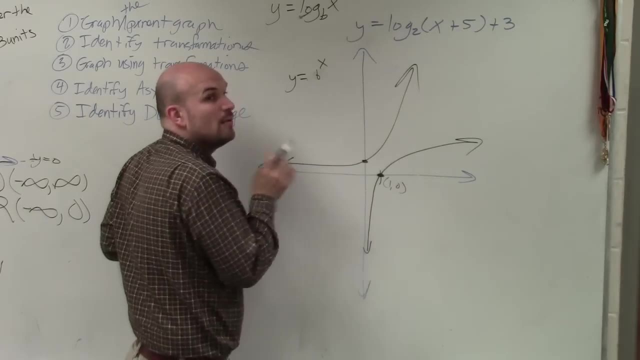 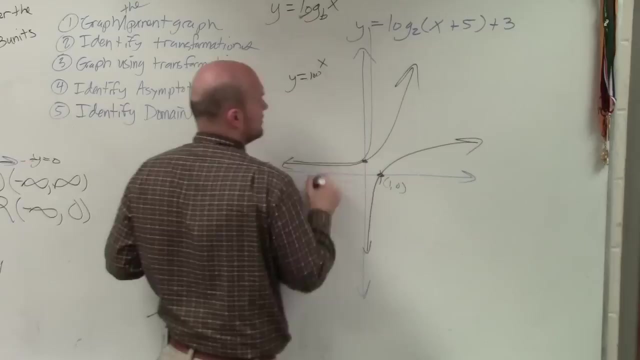 So the graph always crosses at. that graph always looks like this: Always. It's never going to cross at a different value. However, the shape of it could be different, Like, for instance, if I say this is 100, then the graph's going to go like this: If I say that's 1 half, then the graph's: 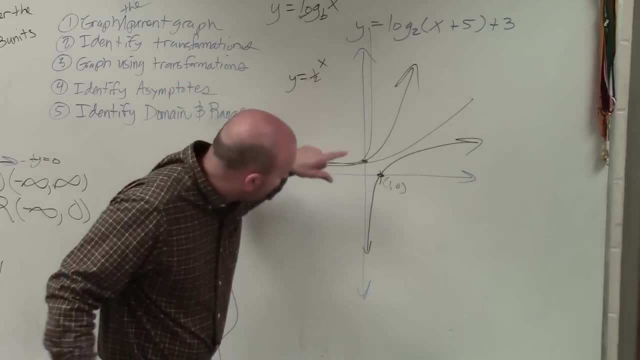 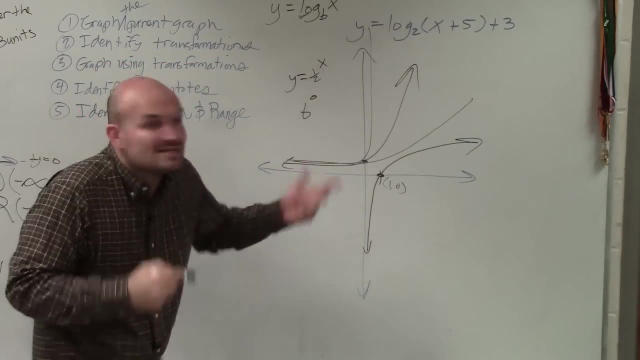 going to go like that, So the shape of it will be different, but it's always going to cross at 0.. Why? Because what is any number raised to the 0?? Narrow power, 1.. So it doesn't matter what b is, It's always going to cross at 1.. 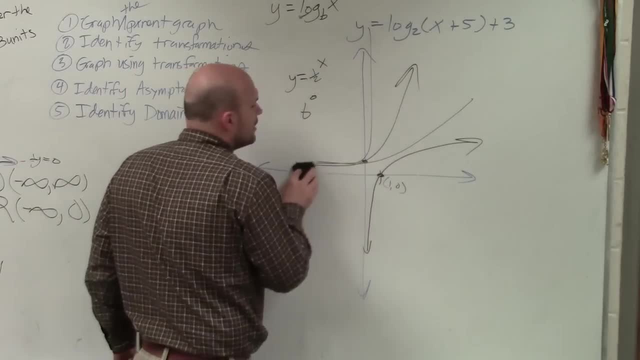 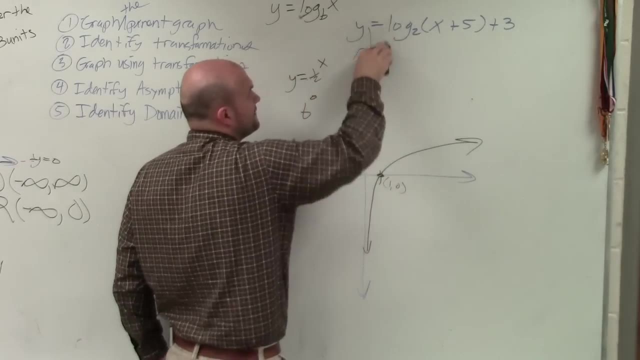 How do you know when to like turn it really sharp? Right now I'm not asking you guys to worry about that with logarithms. So the way that we found out to do if it's really sharp or not for exponential was to use a table of values. right, You plotted. 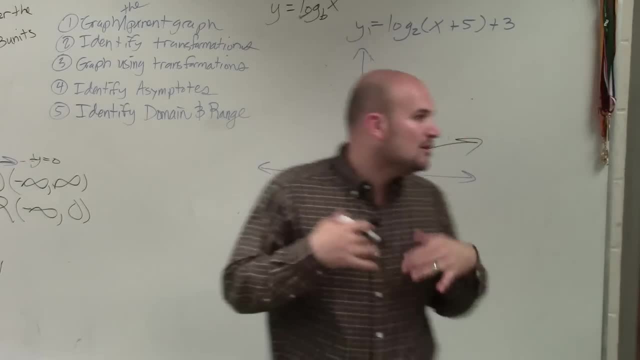 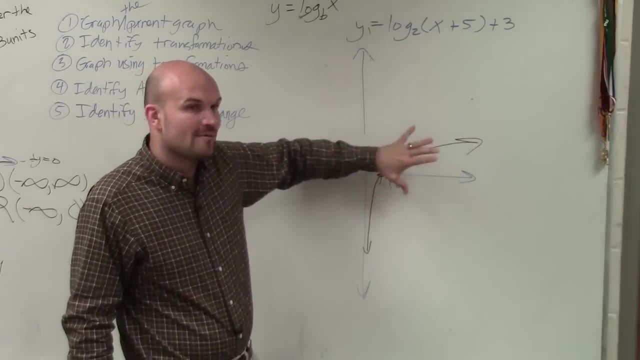 points and that's how we determined if it was sharp or great For logarithms. right now I'm not really concerned. I'm not going to be concerned with the table. I just want you guys to understand what the general format of the graph looks like. okay, That's why I was saying I was kind of easy. 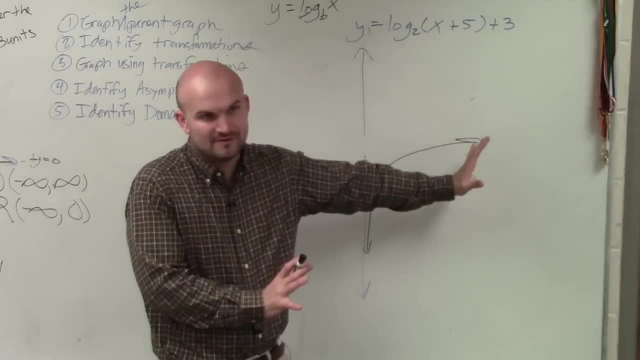 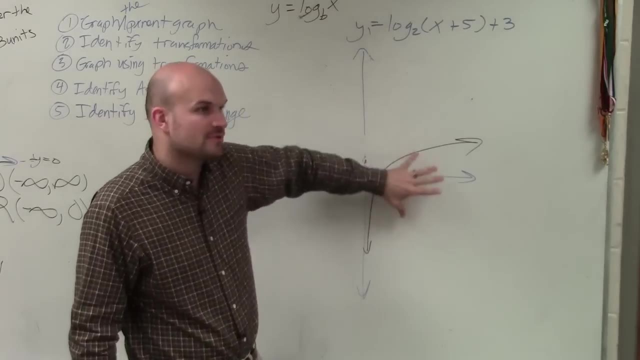 to you guys. I left you off the hook. I just said, hey, sketch what the shape of the graph is, Because once we learn about logarithms, you'll learn how to do a table. But for right now, just know what the shape of the graph looks like and know that it graphs across that 1 comma 0,. 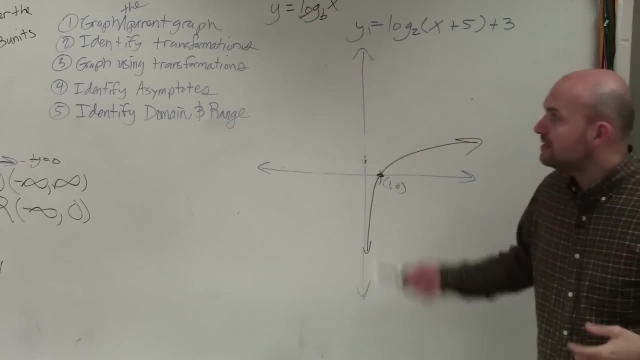 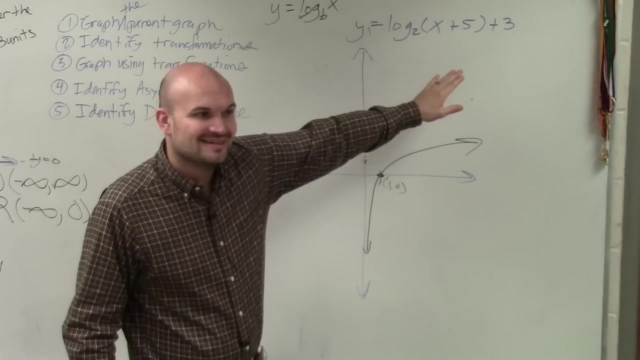 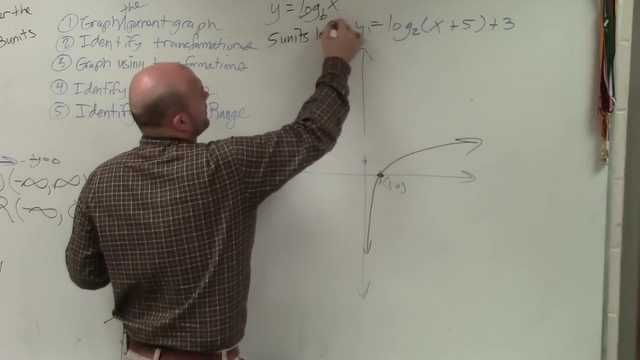 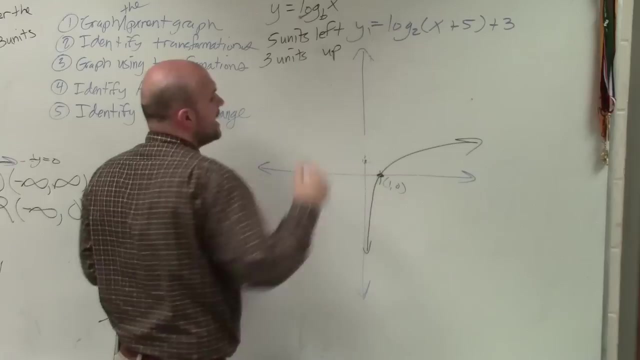 when it's in that format. So now we graph the parent graph. Now let's identify the transformations. So now we have plus 5, which is now going to shift the graph, 5 units left And plus 3 is going to do up 3.. So now, guys, there's only one point I showed you. 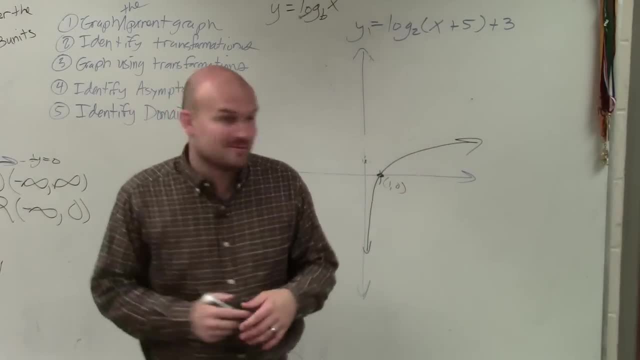 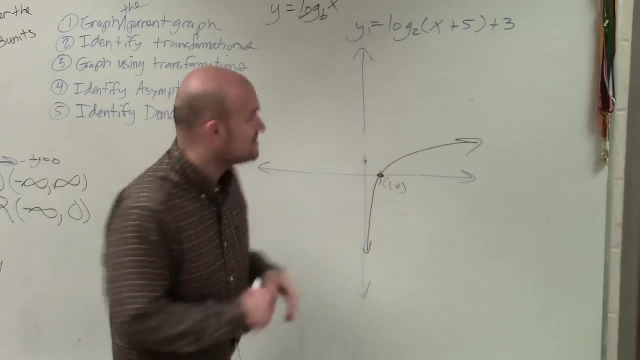 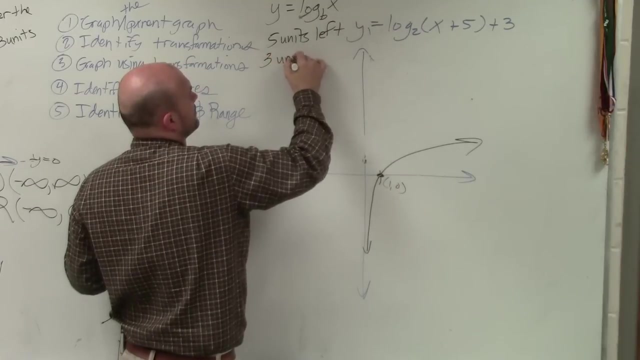 So now we graph the parent graph. Now let's identify the transformations. So now we have plus 5, which is now going to shift the graph, 5 units left And plus 3 is going to do up 3.. So now, guys, there's only one point I showed you for this. 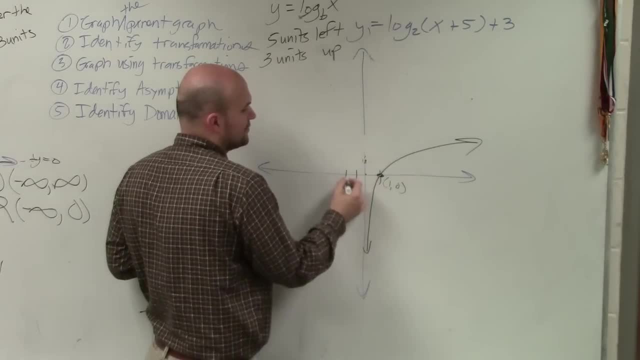 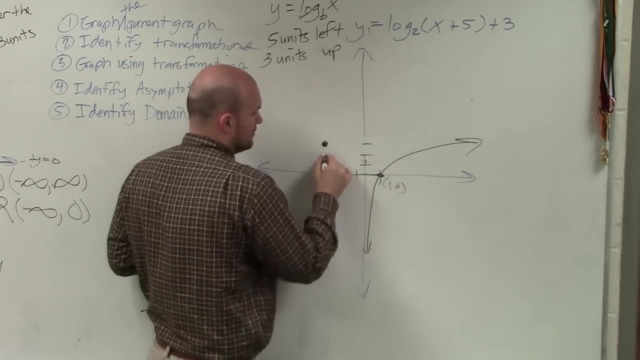 1 comma 0.. So let's go 5 units left: 1,, 2,, 3,, 4,, 5.. And let's go 3 units up: 1,, 2,, 3.. You going to see what I did. 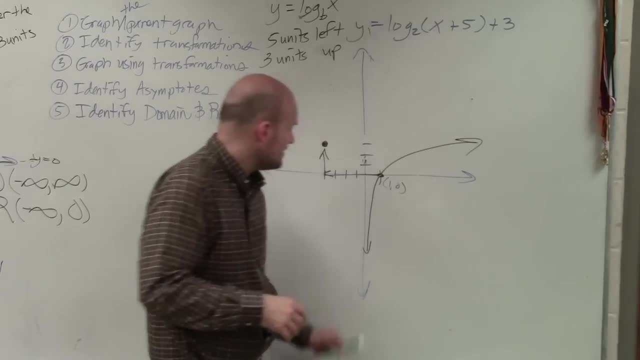 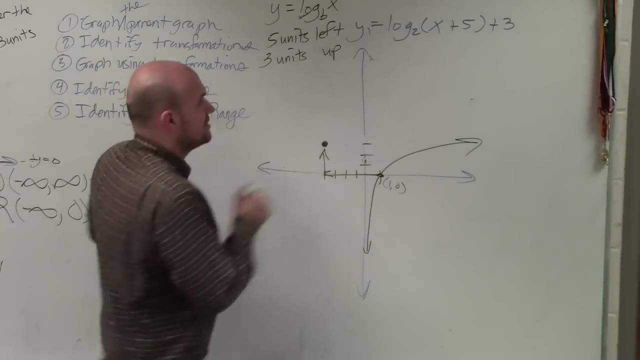 So all I'm doing is taking the exact same graph and shifting it 5 units left and 3 units up. However, it is very important to also identify the asymptotes. When we have an asymptote here, this asymptote is vertical. 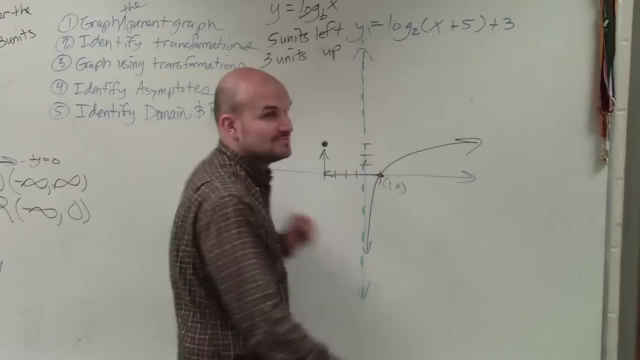 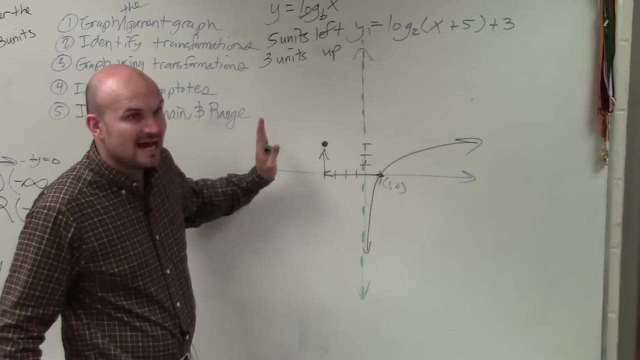 That's where the graph approaches. It approaches a vertical asymptote. Over there it approached a horizontal asymptote. So if I move my graph 5 units to the left, I also need to move my asymptote: 5 units- 5 units to the left. 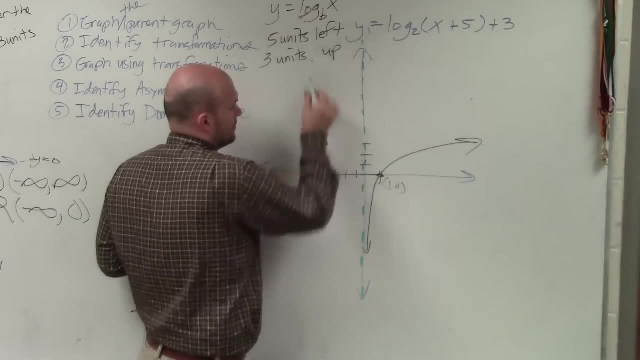 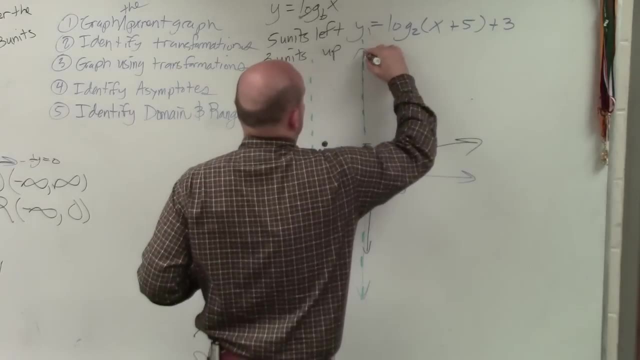 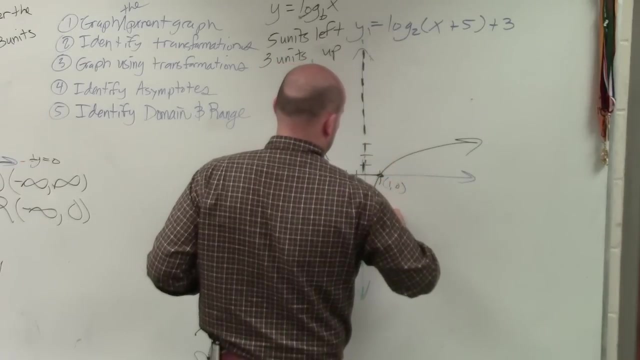 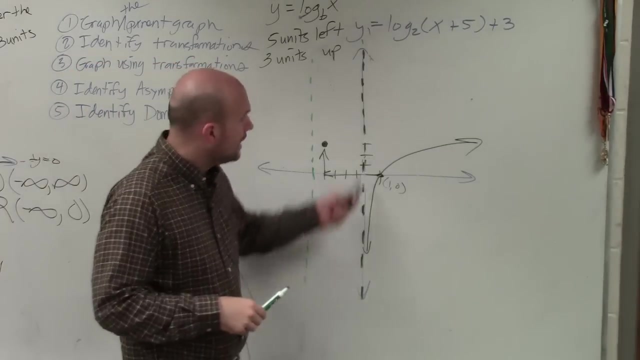 1,, 2,, 3,, 4, 5.. Oh, so the original one is along the 0.. And then when you move it, so it's always going to be along the 0.. I'm sorry, So it's always going to be on the 0.. 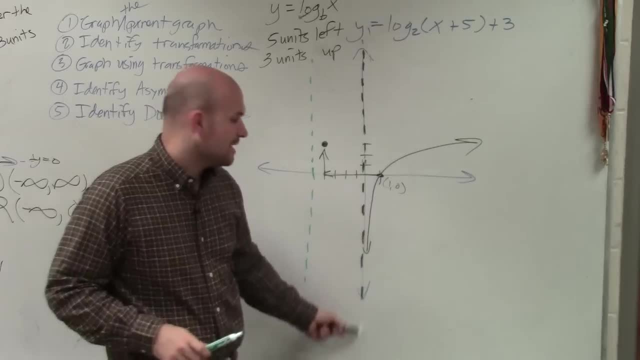 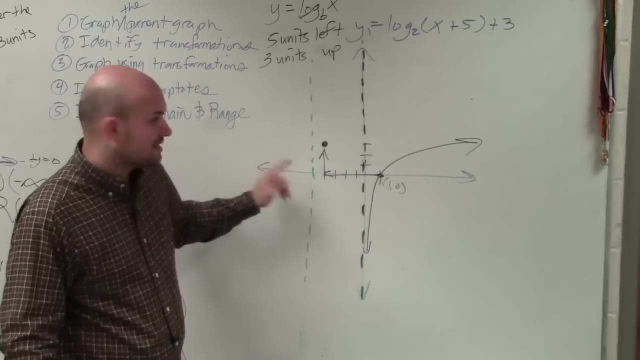 On the y-axis. yes, The asymptote is always at the y-axis, And then on that one, the other graph is on the x-axis. Correct, Yep, Correct Now. so if I'm moving it to 5 units to the left, 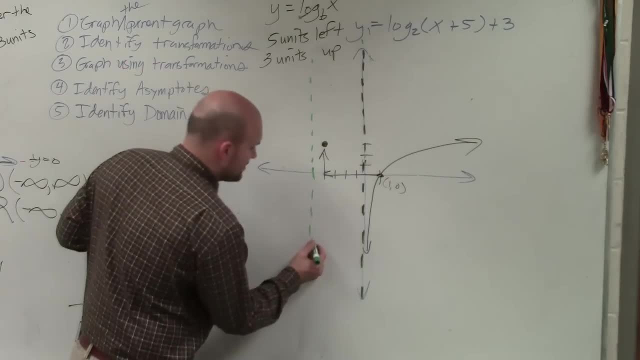 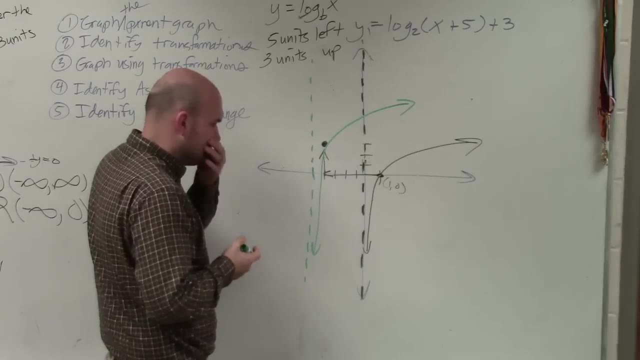 I've got to move the asymptote. I already moved everything else and then I just graph. Now remember, the graph approaches that asymptote, That's the way you like to draw it, But it never touches it And it's not going to touch it. 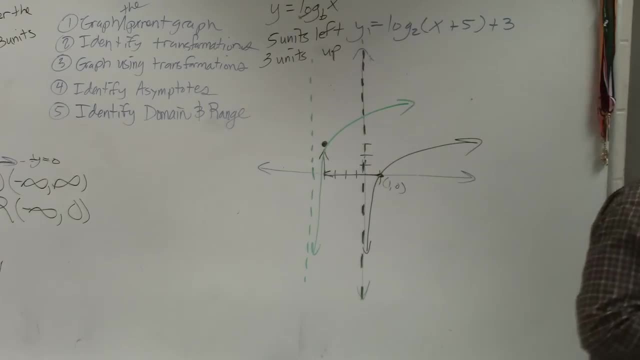 And boom done. Now you've got your graph. That easy. It's a sketch, right? It's not exact. If it was exact, we would have to use a table and figure out how sharp the curve is. It's just a sketch. 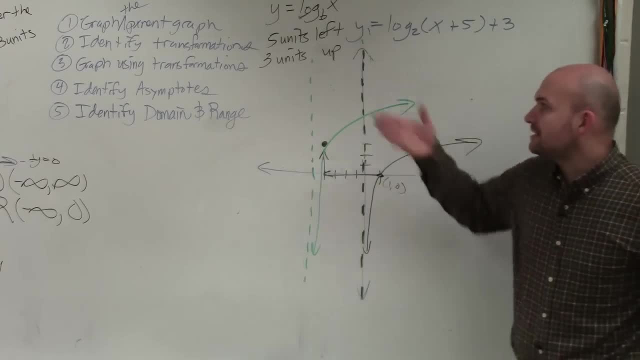 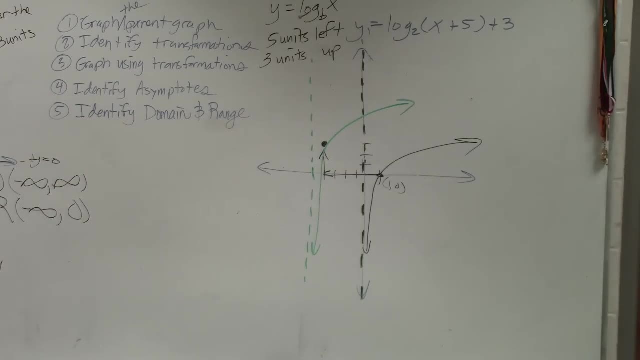 OK, But it's a pretty accurate sketch. Now the last thing is identify the domain and range. So remember, domain was the set of all x values. So here you guys can see that the domain went infinitely that way, infinitely that way. 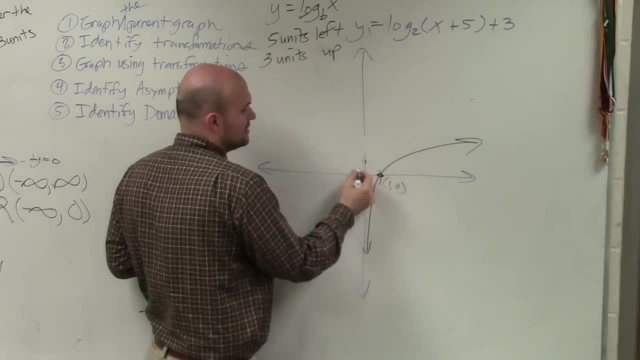 for this 1 comma 0.. So let's go 5 units left: 1,, 2,, 3,, 4, 5.. And let's go 3 units up: 1,, 2, 3.. 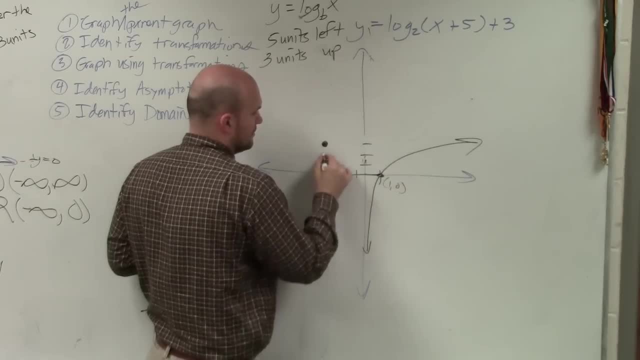 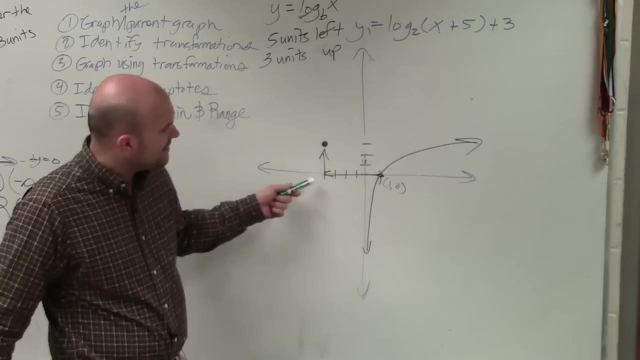 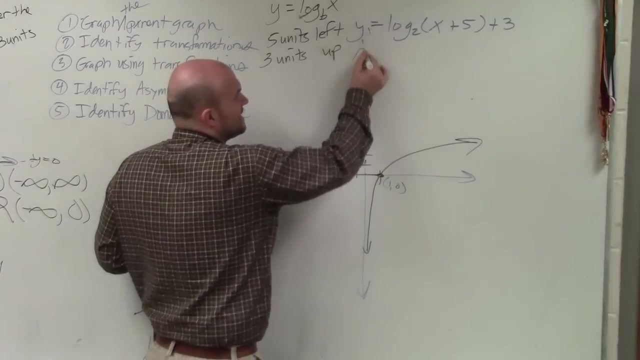 You guys see what I did. So all I'm doing is taking the exact same graph and shifting it 5 units left and 3 units up. However, it is very important also to recognize, identify the asymptotes. When we have an asymptote here, this asymptote. 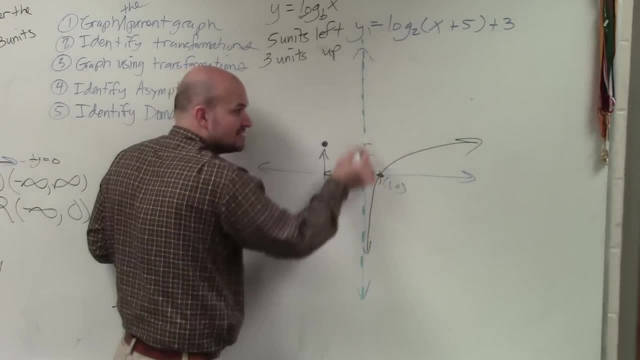 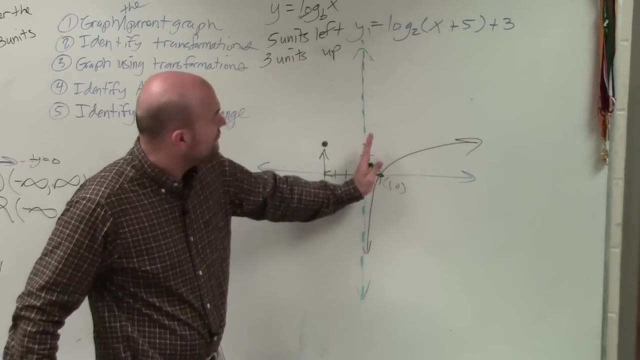 is vertical. That's where the graph approaches. It approaches a vertical asymptote. Over there it approached a horizontal asymptote. So if I move my graph 5 units to the left, I also need to move my asymptote 5 units to the left. 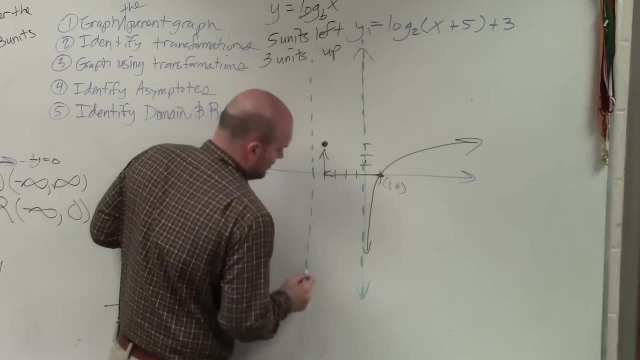 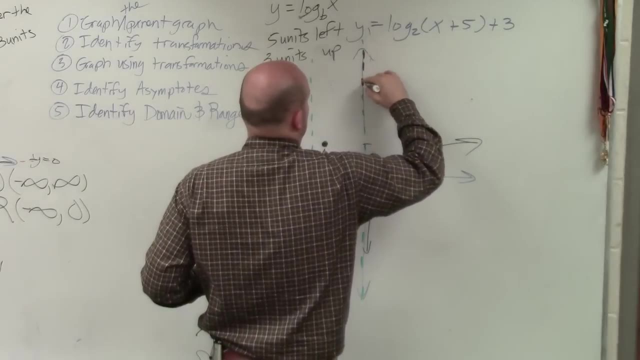 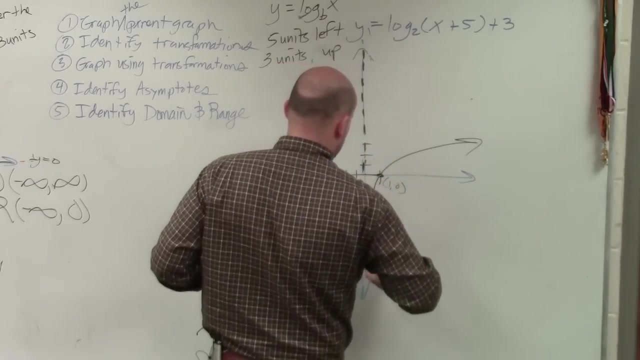 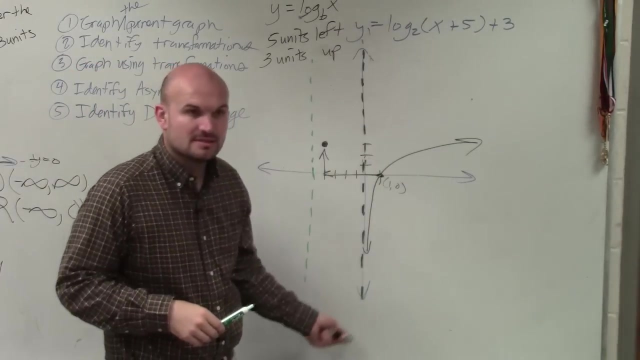 5. I'm sorry, So is that what's going to be on the C-world? On the y-axis? yes, The asymptote is always at the y-axis And then on that one, the other graph is on the x-axis. 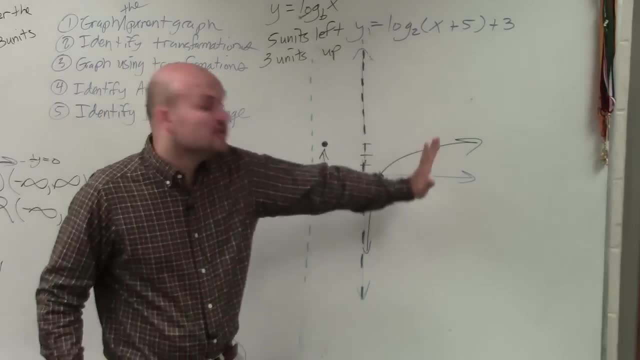 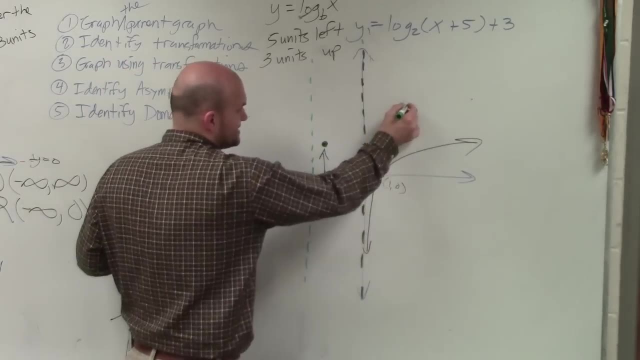 Correct. Correct Now. so if I'm moving it until 5 units to the left, I've got to move the asymptote. I already moved everything else and then I just graph. Now remember, the graph approaches that asymptote. 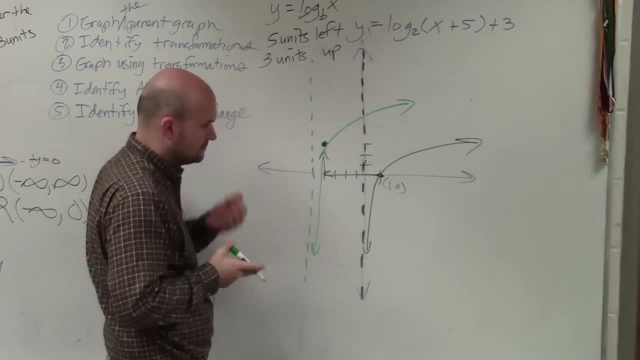 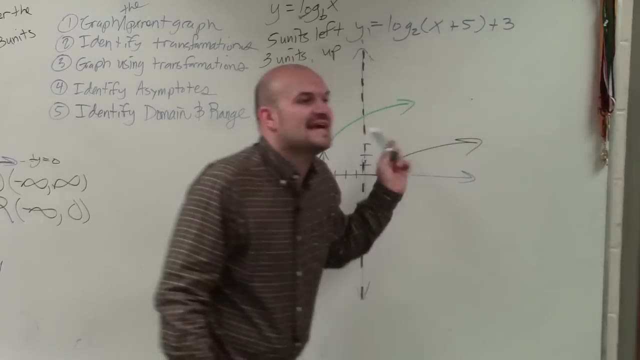 That's the way you like to draw it And it's not going to touch it. And boom, done. Now you've got your graph. that easy. It's a sketch, right? It's not exact. If it was exact, we would have to use a table. 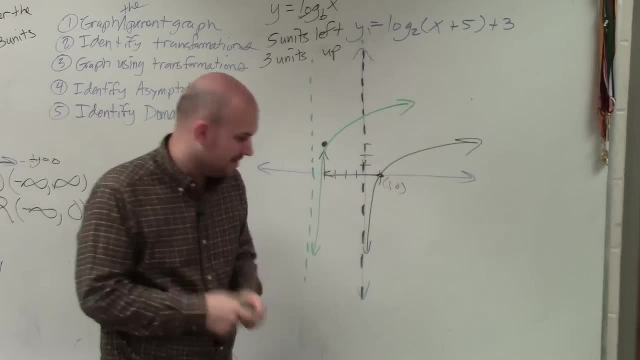 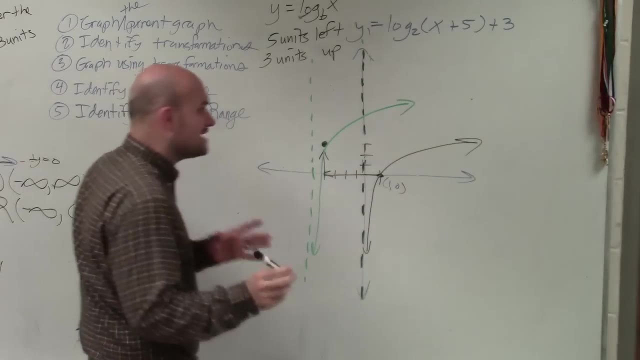 and figure out how sharp the curve is. It's just a sketch, But it's a pretty accurate sketch. Now the last thing is identify the domain and range. So remember, domain was the set of all x values. So here you guys could see that the domain went infinitely. 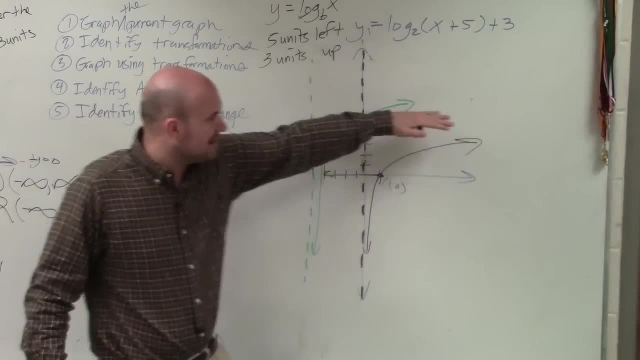 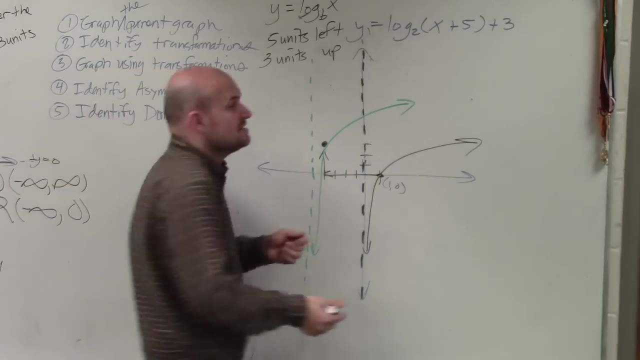 that way, infinitely that way. So the domain: how far to the left does this graph go? Oh, negative, 5.. 1,, 2,, 3,, 4, 5.. Yeah, it's only going to go as far as the asymptote. 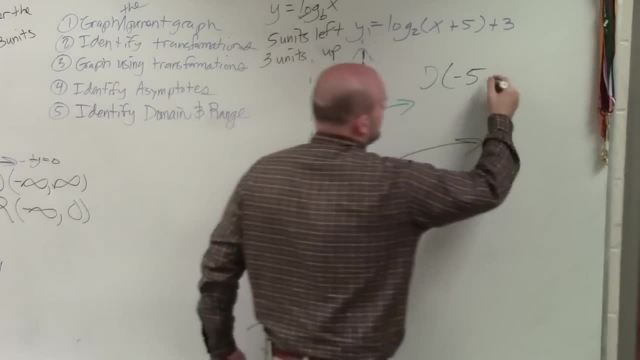 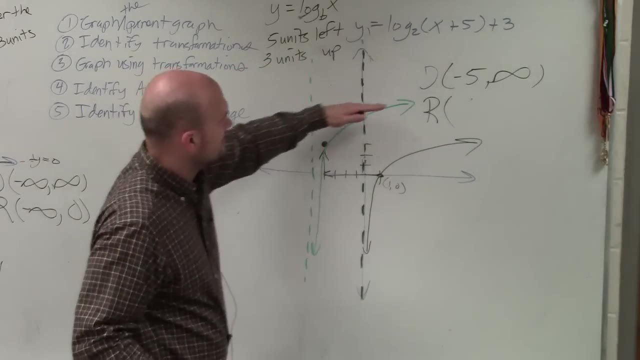 So the domain is from negative 5.. Well, how far to the right does it go? Infinity Range. How far low does this graph go? It's at negative infinity, Negative infinity. How far high is it going to go? Negative infinity, I mean infinity.